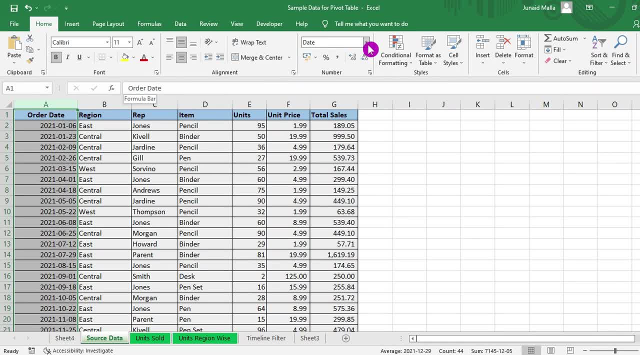 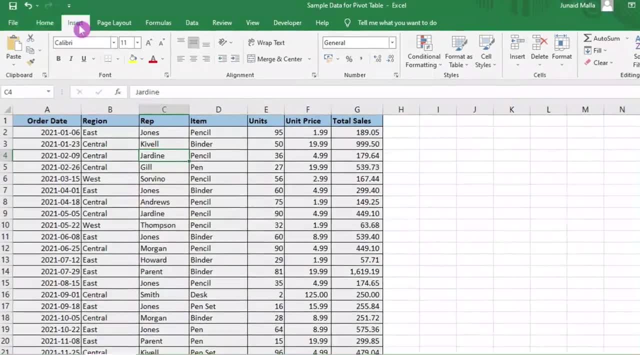 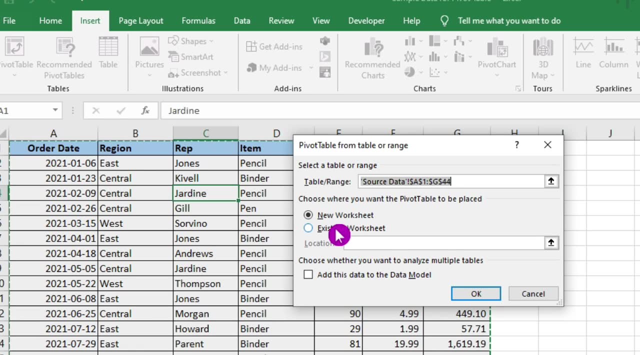 first of all, you will ensure that the column which contains the date data is in the date format. then what you will do is that you will click anywhere in your data, then click on insert tab, click on pivot tables. then you can either choose a new worksheet or you can select the existing worksheet. 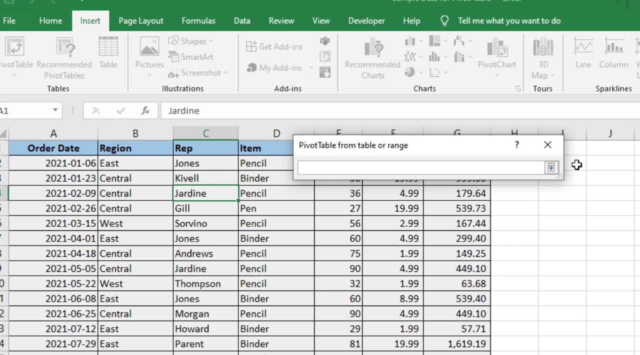 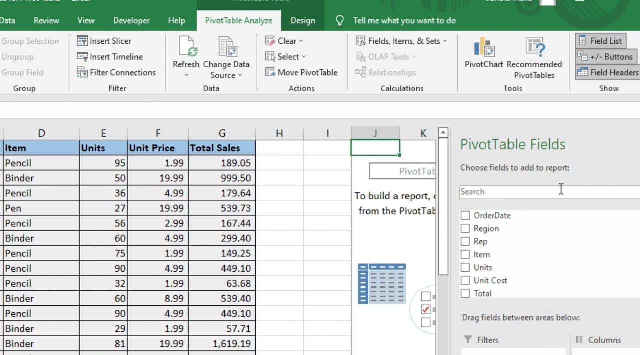 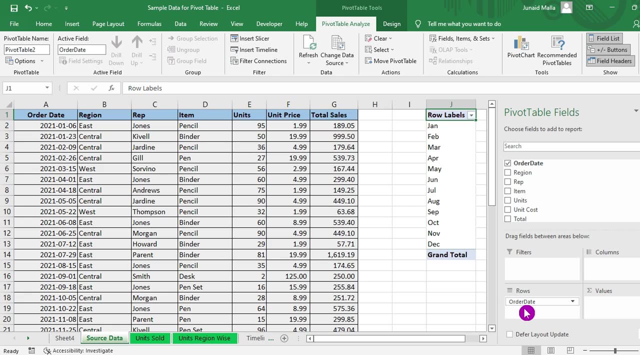 i will select existing worksheet here, then i will select a location for the pivot table, then i will click on ok. and here what you have to do is that you have to drag the order date. you have to drag the order date field in the rows box and you have to drag the total sales field in the values box. and here you have to ensure that. 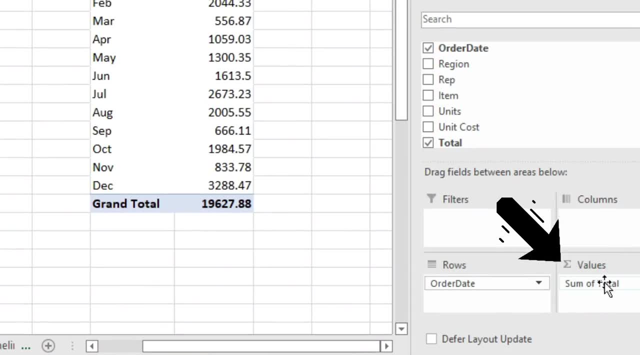 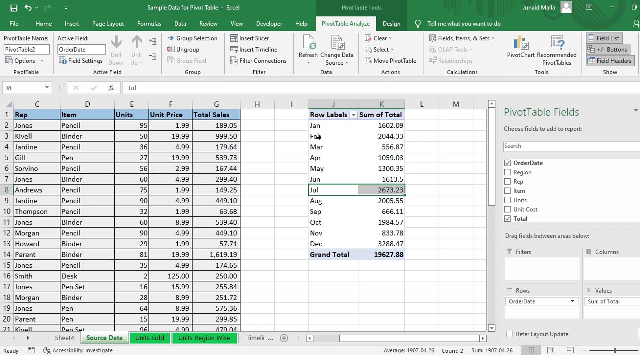 the values field calculates some, because there are other options also. you can calculate average or count also, so make sure that it is sum of sales here in this, in the values field. here you have your data month wise. now what if you want to calculate sales data quarter wise, what you will? 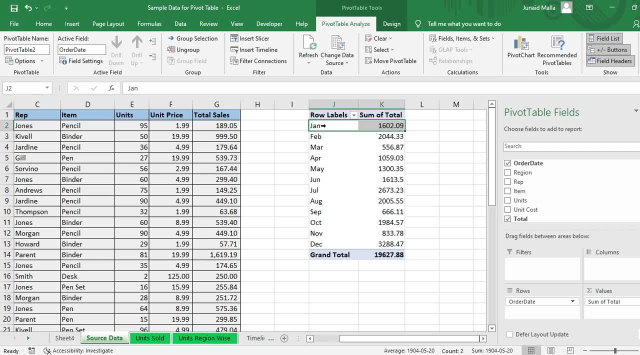 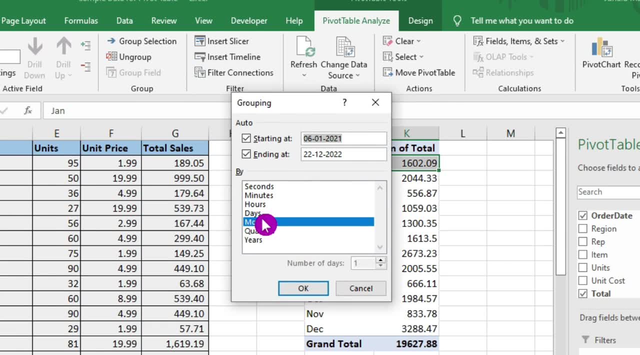 do is that you will click anywhere in your data tab and click on calculate total sales figures. your in the month field. then go to pivot table analyze. then click on group selection and select quarter. here you will select quarters. here then you can choose a starting date and an ending date. 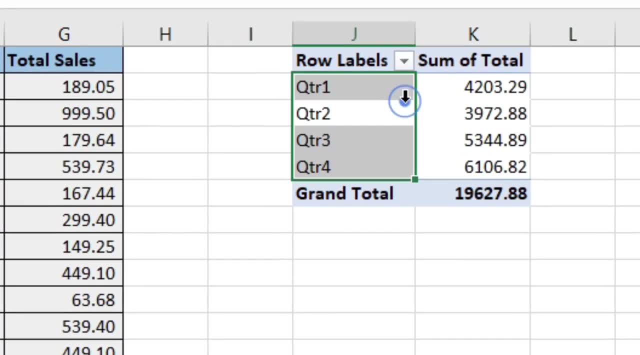 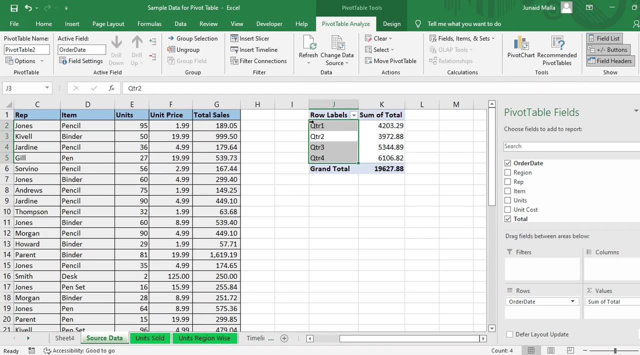 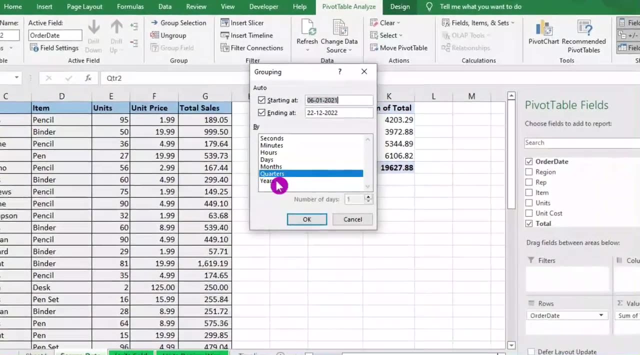 for the pivot table data. then click on ok and here you have your data by quarters. now what if you want to calculate the sales data by year? then add quarter as a quarter, as a subgroup. you will click on group selection here. then select the year field, also click on ok and here you can see that in the 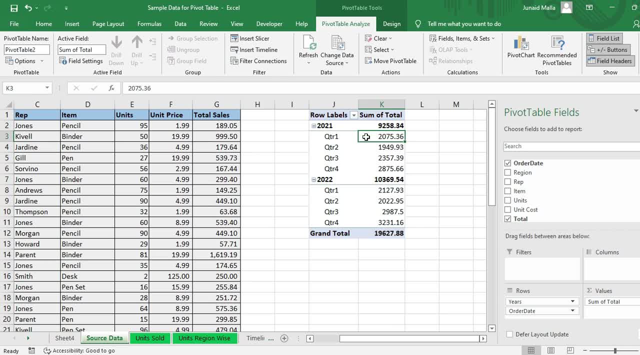 year 2021, this amount is the sales for quarter first. this amount is the sales for quarter second, and so on and so forth. similarly, for the year 2022, this amount is the sales for quarter one. this amount is the sales for quarter two, three, and so on and so forth. so this is how you can. 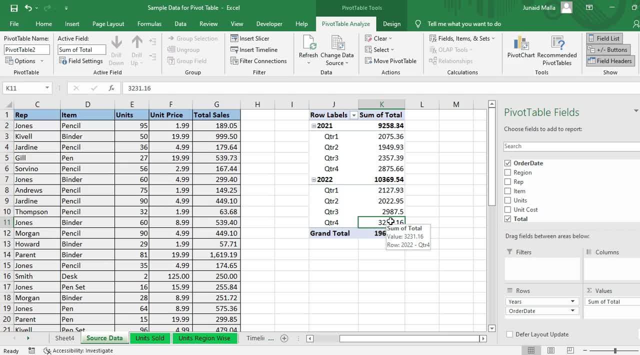 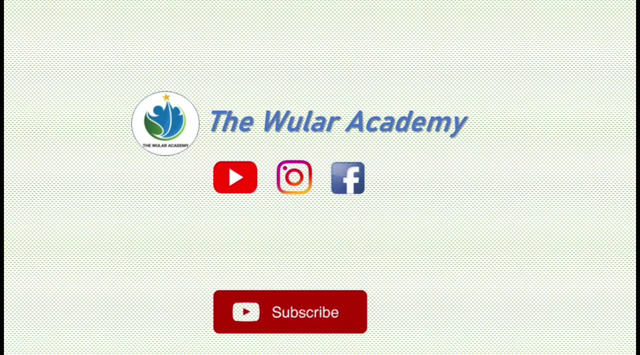 group items or summarize sales by year, quarter or month. i hope this video was helpful. if you like the video, please give it a thumbs up, keep supporting, subscribe the channel. thanks for watching.